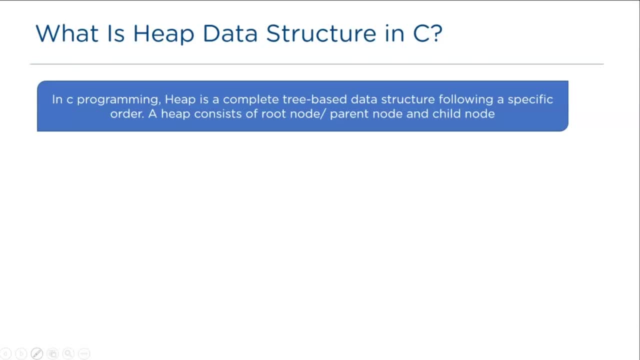 for a tree. similarly, a root node is very important. in a heap, The element of a root node is always greater than or equal to the other tree nodes, Or it can be smaller than or equal to its child node. Suppose we have an array of elements: 7, 5,, 6,, 2 and 3.. And 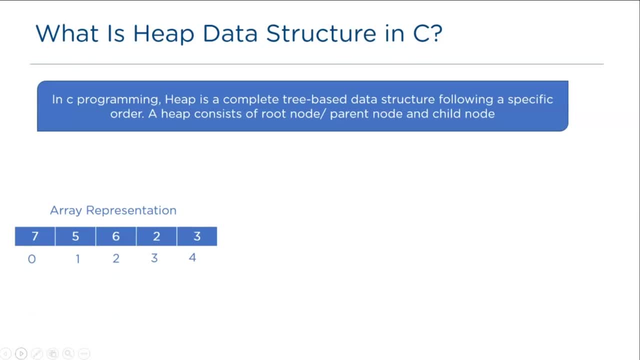 the index starts from 0 up to 4.. So heap is a tree based data structure. As you can see, the highest element is our root node, followed by the children nodes. Node element 5 and 6 are the child nodes of node. 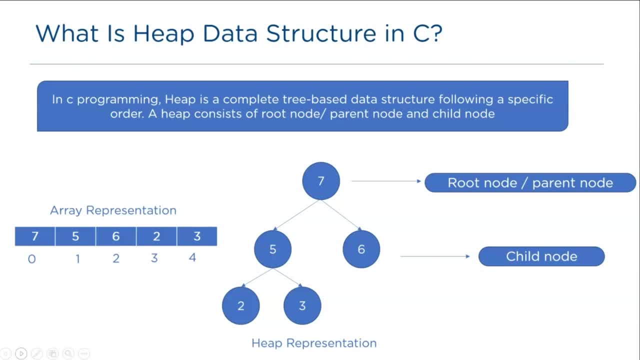 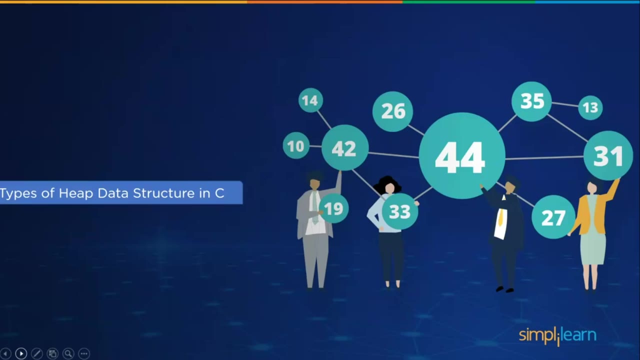 7. Whereas node 5 is a parent node of 2 and 3.. And if it is required to insert a few more elements in a heap, it starts inserting from left to right And let the root node index be 0 and goes up to the elements present in a heap. Now we know what a heap data structure. 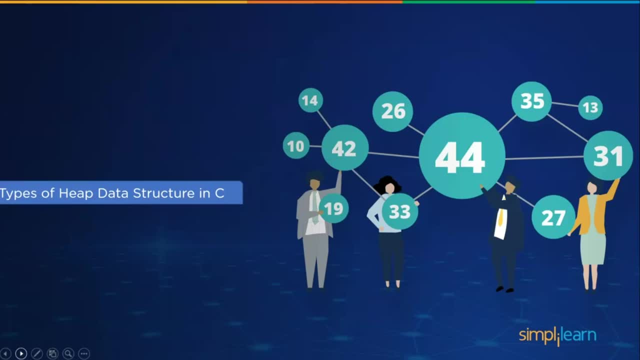 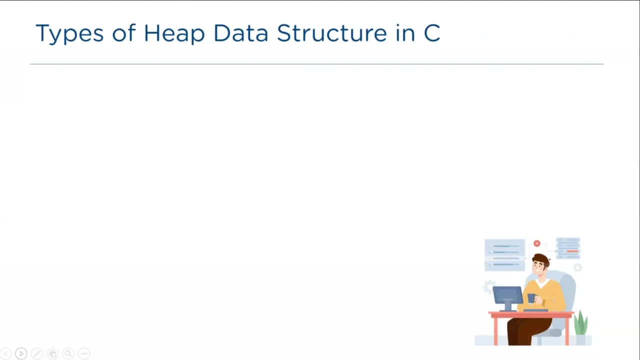 is And why heap is used in C programming. Let's move ahead and understand the types of heap data structure in C. There are two types of heaps: max heap and min heap. In a max heap, the elements of the root node must be greater than or equal to the elements of its children's node. Now let's 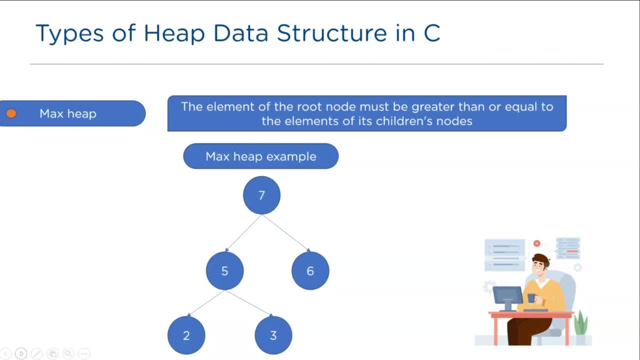 see its example. In this particular example, 7 is the largest element than other elements in the node. So when you see towards down, the heap parent node element is greater than its children node. For example, root node 7 is greater than 5 and 6 and 5 is greater than its children. 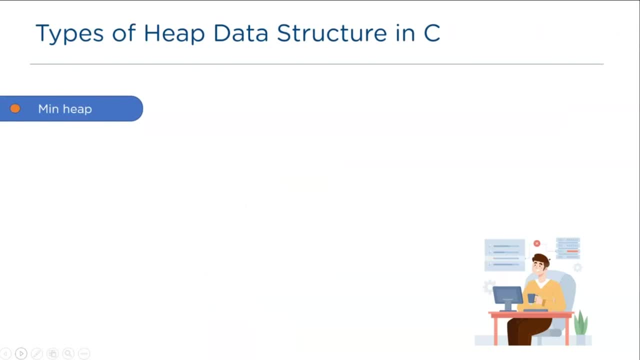 node 2 and 3.. Min heap is just opposite of max heap. The root node element of a min heap is lesser than or equal to its children. node, For example, 2 is lesser than all other nodes in a heap. The parent node 3 is lesser than its children node 6 and 7.. 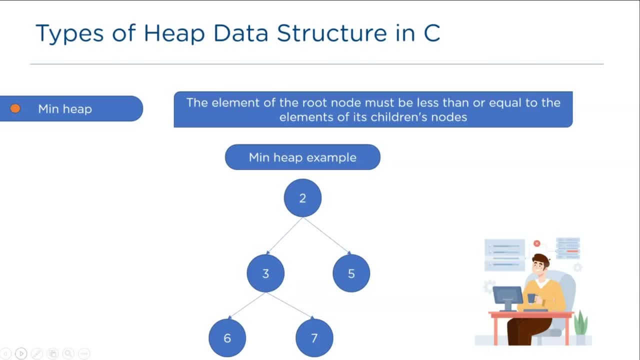 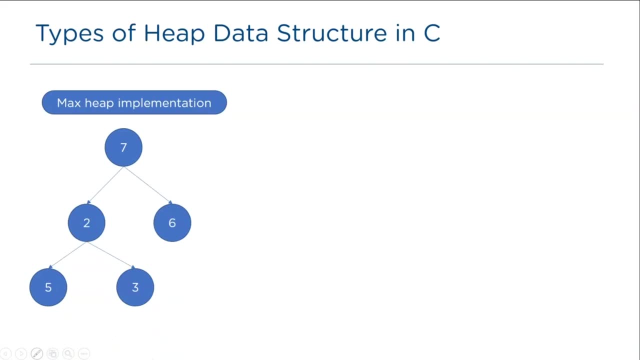 So I think you understood max heap. So let's move on to the max heap implementation. Here we have an example. The heap elements are 7, 2,, 6,, 5 and 3.. Now look at the steps. 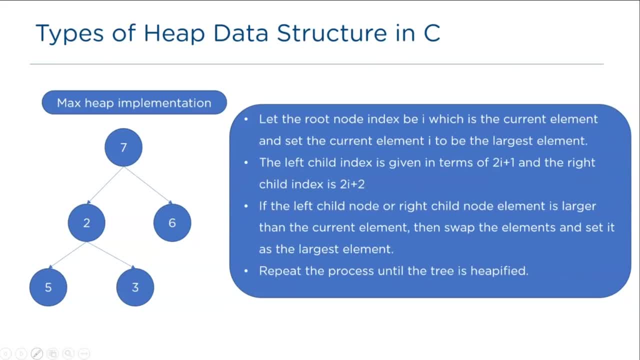 to implement a heap, Let the root node index be i, the current element, and set the current element i to be the largest. In this given example, a parent node of 5 and 3, which is 2, is lesser than its children node. 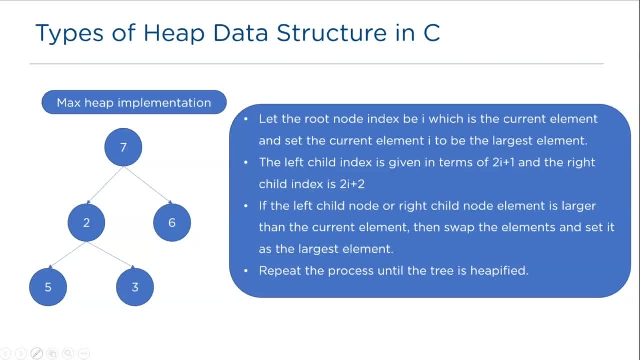 So heapify the heap. The left child index is given in terms of 2i plus 1 and the right child index is 2i plus 2.. By considering this example, the index of node 2 is 1.. So by 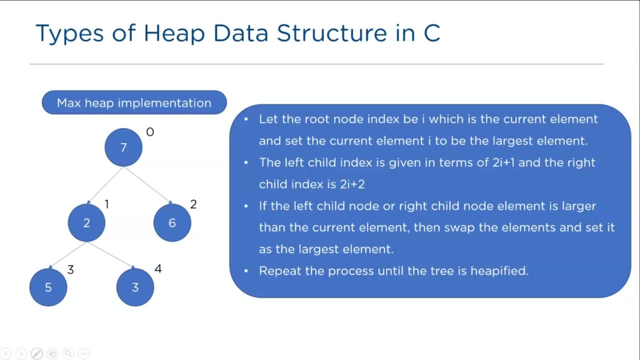 calculating the left child index: 2i plus 1, whereas i is equal to 1. So 2 into 1 is equal to, 2 plus 1 is equal to 3.. Swap the element with the index node 3.. That is swap the elements. 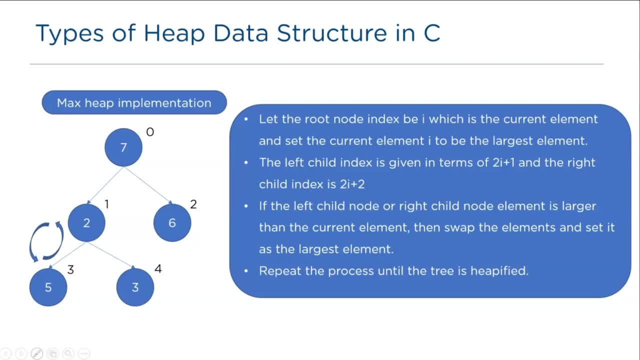 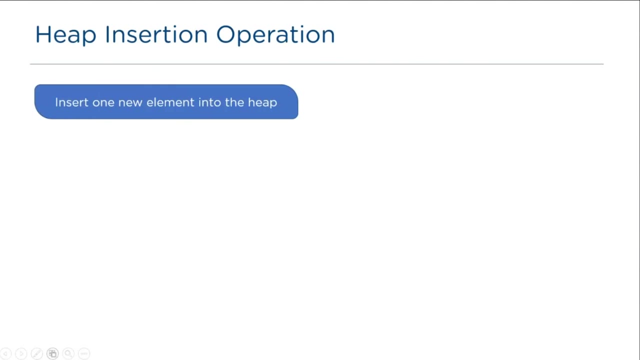 2 and 5.. So now the parent node is greater than its children node And finally, the tree is heapified. Now let's have a look at the heap insertion operation. Let's insert one new element into the heap. For example, if the element is 7 to be inserted, 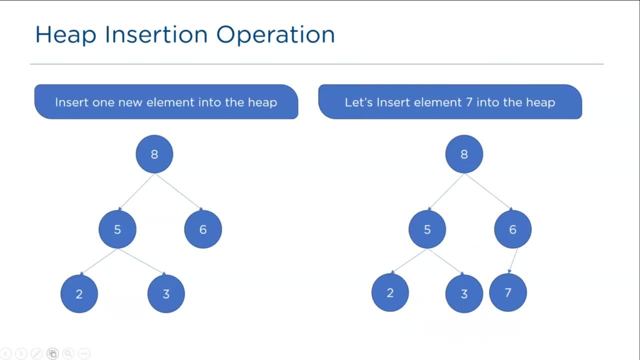 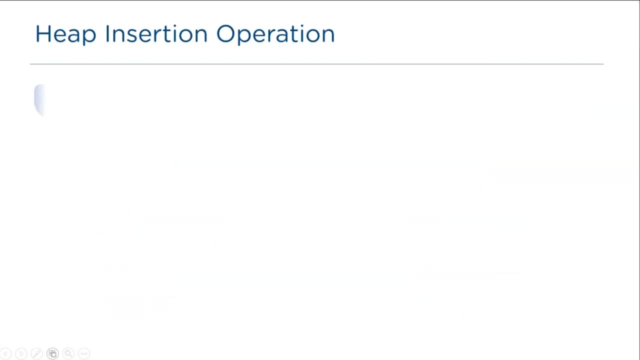 then it will be inserted from left to right at the bottom of the heap, Since the parent node element is less than its child node, That is, 6 is less than 7.. For this all the so, we must happy 5.. So the next step is to happy 5 the tree by swapping the elements. 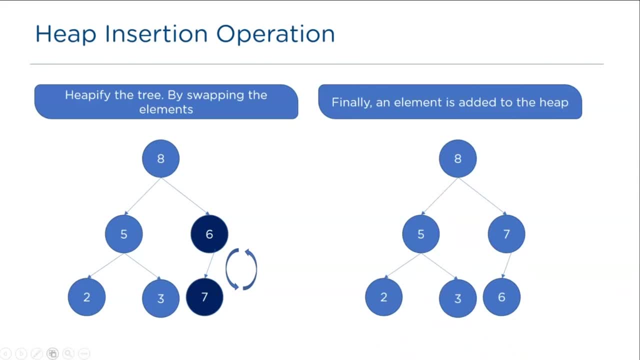 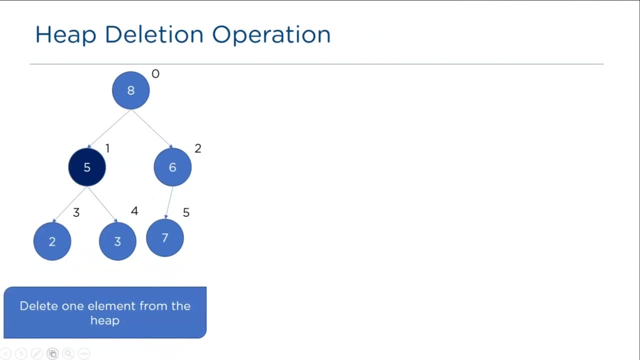 And finally, the element is added to the hip. Next is a hip deletion operation. Suppose we want to delete one element from the hip. So let's consider element 5 to be deleted. and to delete element 5, swap the element with the last node, element 7.. 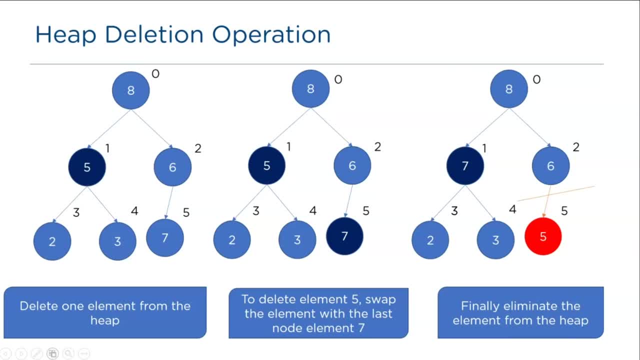 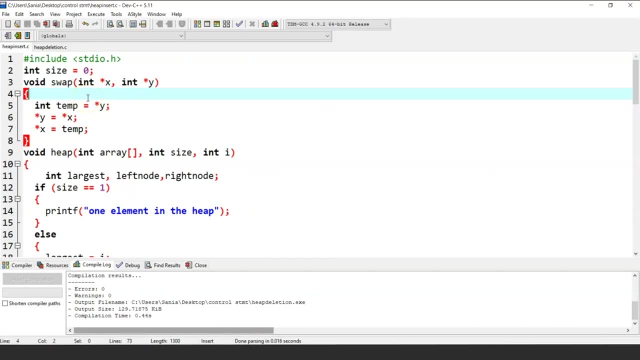 And finally remove the last element from the hip. Now let's run this simple program using hip data structure. So in this program we are going to insert and happy 5, the hip elements To organize the data of a hip max. we have swap function in which we are going to swap the elements between parent. 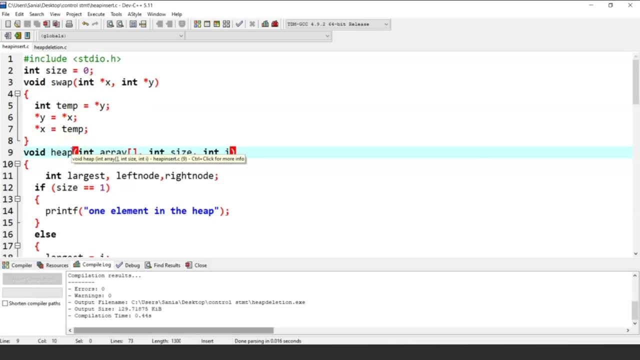 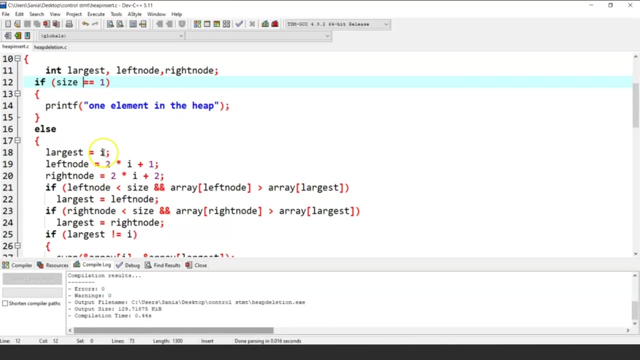 node and child node Following. we have a heap function. It first checks whether the size is equal to 1.. It means there is only one element in the hip, Else it will set the current element, i, to be largest. As we discussed before, the left node index is given in terms of 2 into i plus 1 and right node. 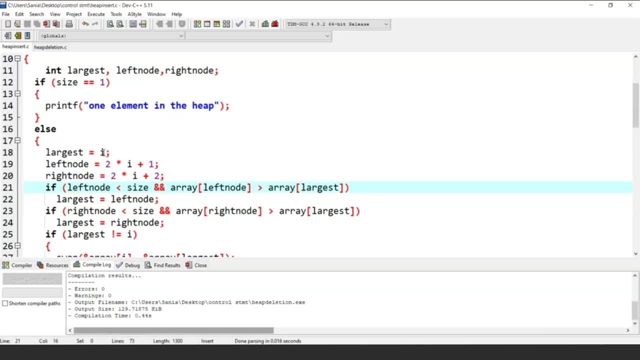 is 2 into i plus 2.. And if left node is less than the size of hip and greater than the largest, then it will set the left node to be largest. Similarly we do for the right node, And then we have an insertion function to insert the elements in the hip. 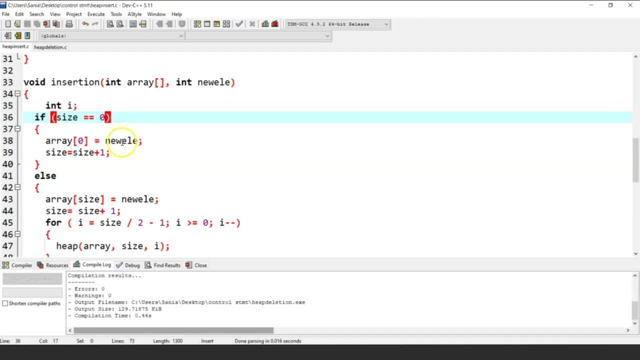 Using if condition, it will first check the size of hip. If it is 0,, then array index of 0 will be the new element And then increase the size by 1.. Else array size is new element. So once we insert the element into the hip, 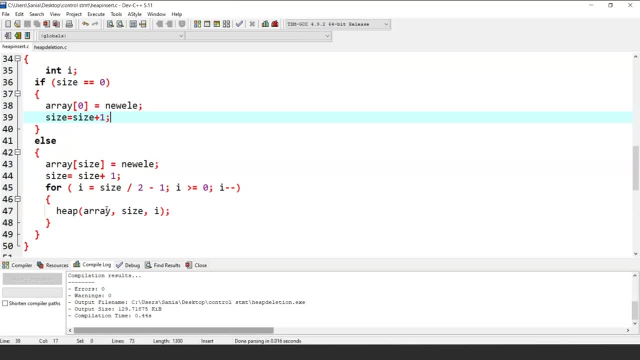 we are calling a heap function to organize the data. That means to happy 5.. And once the data is happy 5, we have a print function. It will print all the array elements And then, inside the main function, we are giving the values to insert the elements and the 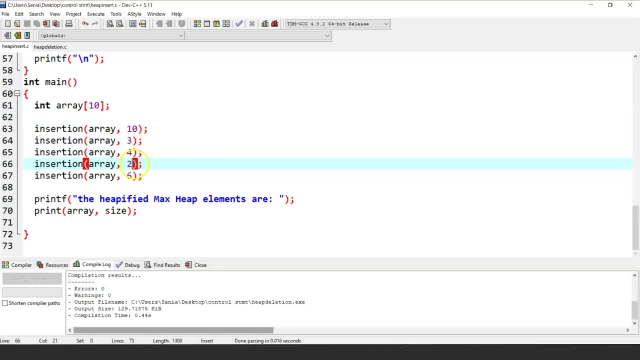 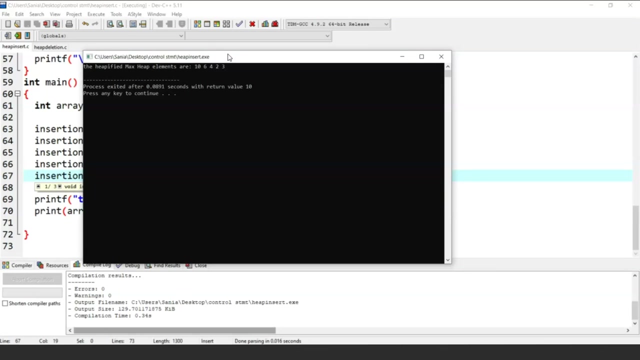 are 10,, 3,, 4,, 2, and 6.. And finally, it will print the happy 5 max-zip elements. So now let's run the program and see the output. As you can see, the happy 5 elements are 10,, 6,, 4,, 2, and 3.. So now let's try to insert one more. 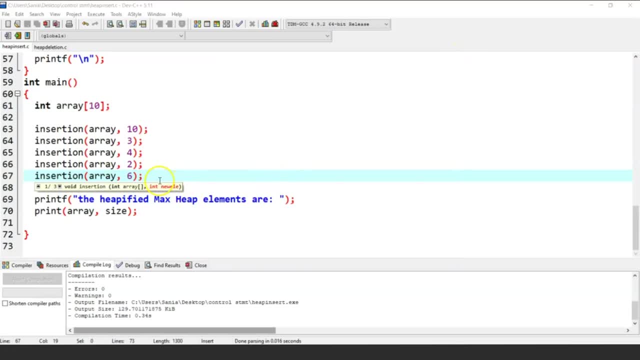 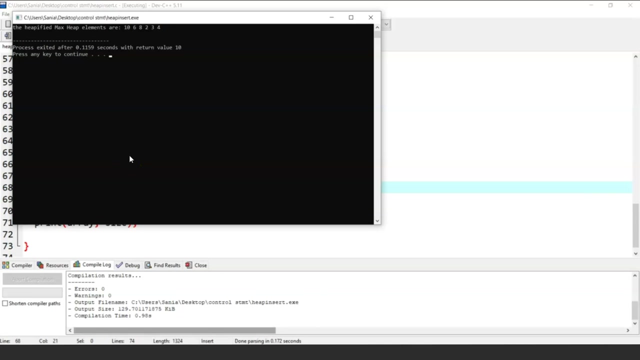 element and see the output. And, lastly, let's run the program and see the output, And finally the and save the output. So let's insert the element 8.. Save the program and run. And here we go: The element 8 is successfully inserted. 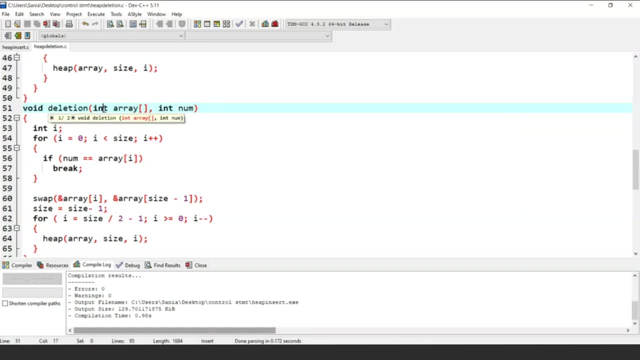 In our next program let's try to perform deletion operation. So let's try to delete one element from the heap. So for that we have a deletion function. If number to be deleted is equal to the array of index, then swap the element with the last node.